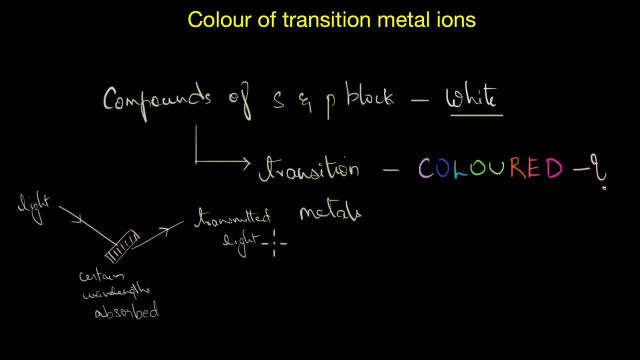 to the color that got absorbed gets transmitted. For example, plants appear green because they mostly absorb red light and some blue light, while the green light gets reflected. Now this absorption of light in the visible or the UV region occurs due to the changes in 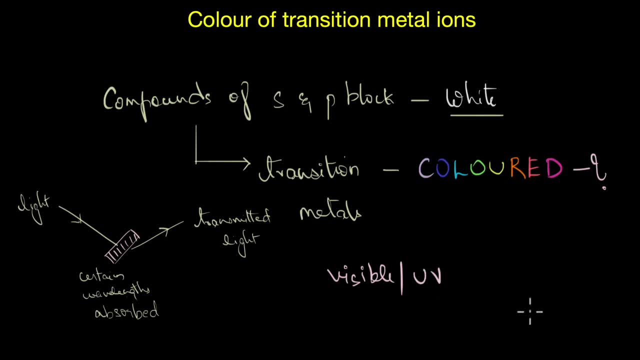 the electronic energy, That is, the energy that is associated with the absorption of light. So the absorption of light in the visible or the UV region occurs due to the changes in the electronic energy, That is, the energy that is associated with the absorption. 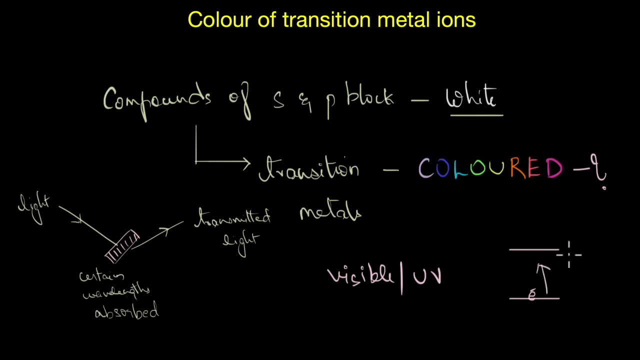 of electron from one energy level to the other. Now, usually the energy jump is so large that the absorption lies almost always in the UV region. But in some cases it is possible to obtain small jumps in the electronic energy which usually appear as absorption in the 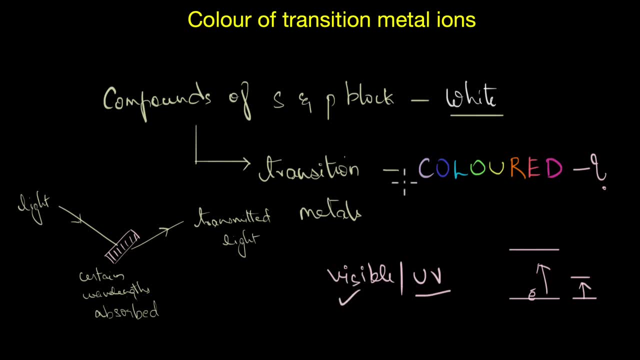 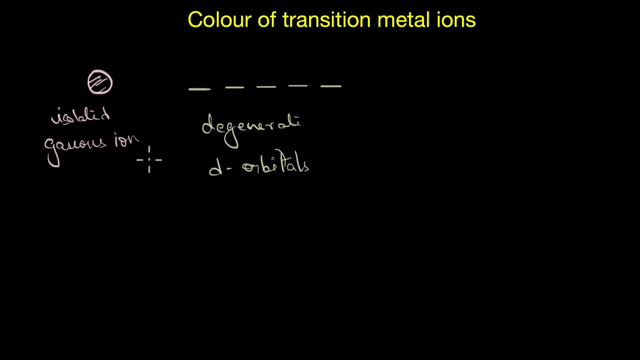 visible region. Now things take an interesting turn when we talk about ions with incomplete D or F orbitals. You see an isolated gaseous ion of a transition metal that is free from any external influence, has 5 degenerate D orbitals. That is all the orbitals here are. 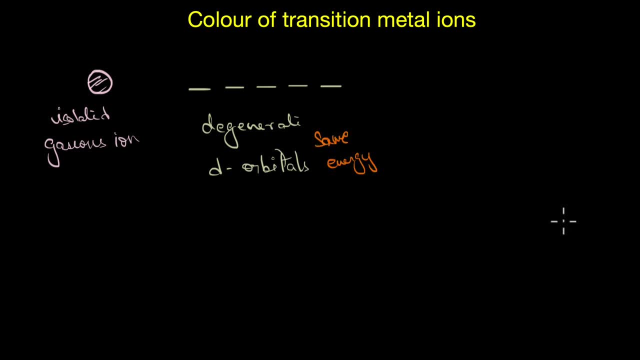 of same energy, But in reality these ions are not really isolated. They are usually surrounded by solvent molecules. For example, in the case of copper sulphate, hydrated copper sulphate, where copper ions are coordinated or associated with 5 water molecules and this ion and this complex is 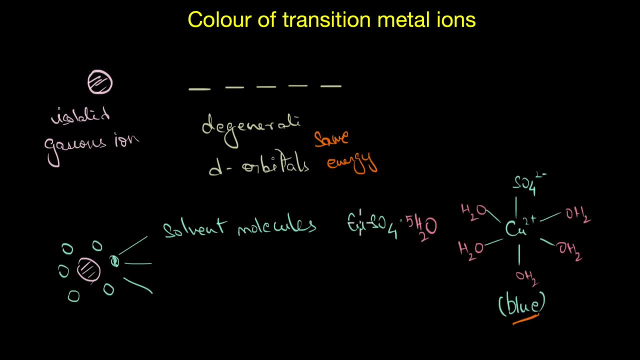 actually blue in colour. So here, as you can see, the ions can be coordinated with solvent molecules. It can also be coordinated by other ligands in complexes like FeCn6, 4- or even other ions in crystal lattices, like in the case of MnO4-. 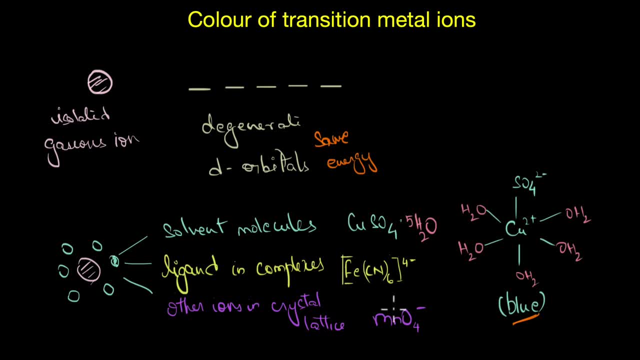 So, as you can see, the ions are not actually isolated, but surrounded by different types of ions, depending on whether it is in a crystal lattice or in a solution or in a complex, And these surrounding molecules will have some kind of effect on the transition metal. 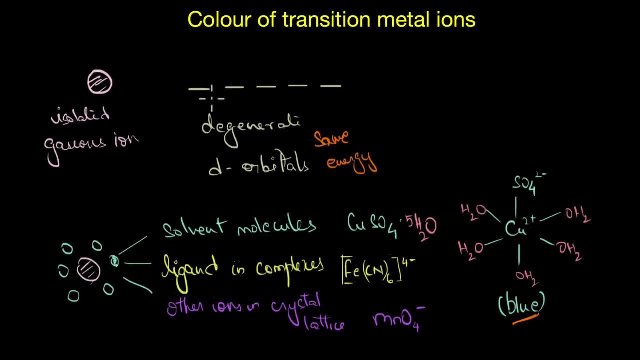 ion right. Of course, The surrounding groups affect the degeneracy of the D orbitals and, as a result, the D orbitals split into two groups, Two groups of D orbitals of two different energy levels. Because of this, we can easily promote an electron from one D level to the other D level. 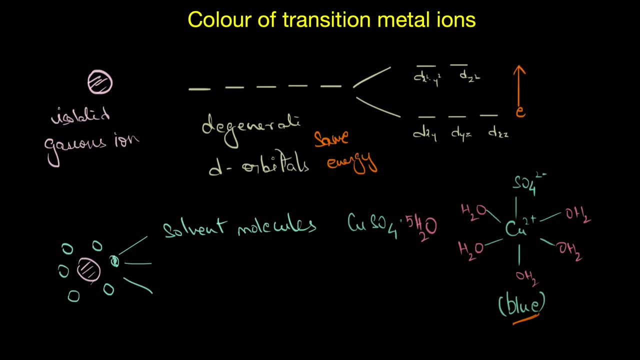 of higher energy. As the energy difference between the two D level is not very high, the light is absorbed in the visible region. Now the colour that is transmitted depends on how big the energy difference is between the two D levels, And this further depends 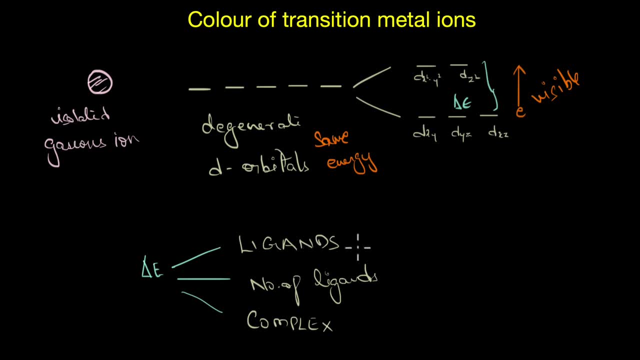 on the nature of the ligands- whether it is a strong ligand or a weak ligand- number of such ligands and the type of the complex. Now, we cannot discuss more about these factors in this particular video, But to give you 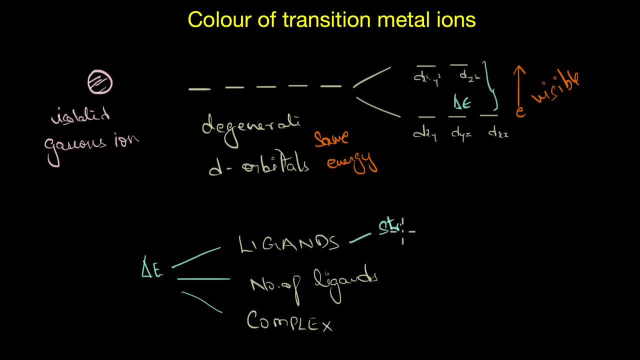 an overview: if we have a strong ligand, then the D energy levels would split more and therefore the delta E would be larger, Whereas if we have a weak ligand, the delta E would be smaller And, depending on this energy difference, we get the corresponding colour. For example: 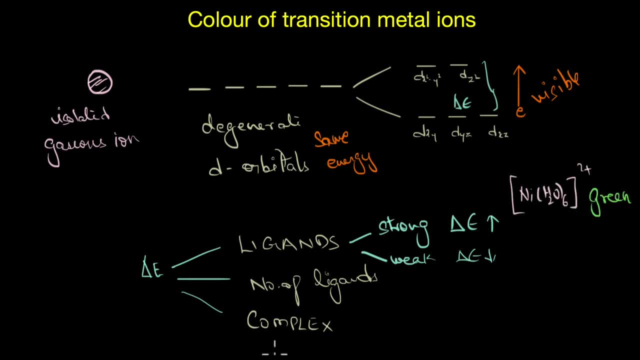 NiH2O6 is green and green is blue, Whereas NiNO26 would be brown- red in colour. So, even though we have the same metal ion, which is nickel, depending on the type or the strength of the ligands it is attached to, the nickel complexes can get different. 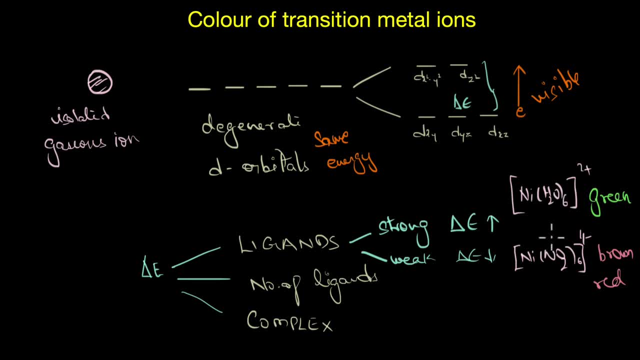 colours. Now, what makes a ligand strong or weak is something that we cannot cover in this particular session, but will be covered in great detail in your next unit on coordination chemistry. Ok, So now let's understand that ligands can be classified into strong and weak, And depending 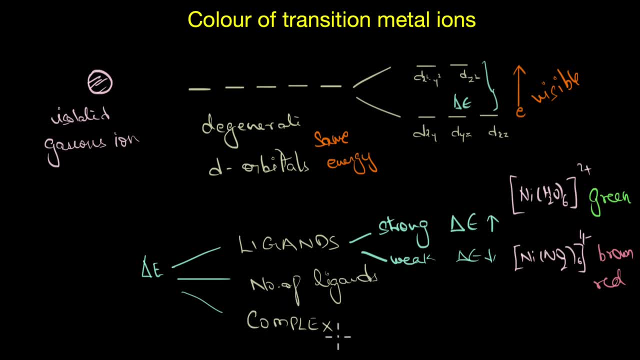 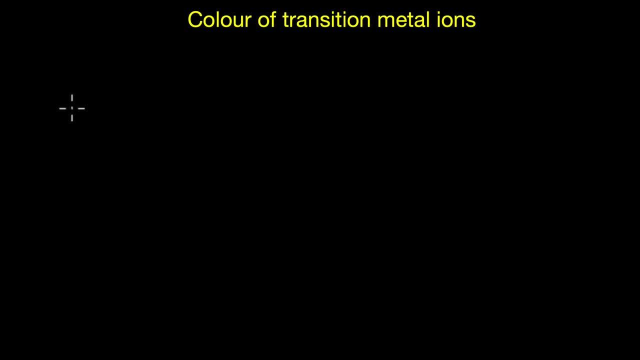 on the strength of the ligands, the number of ligands and the shape or the type of the complex that is formed. colour shown by a particular ion can vary. However, we do have some white coloured compounds of transition elements too, For example zinc sulphate and.